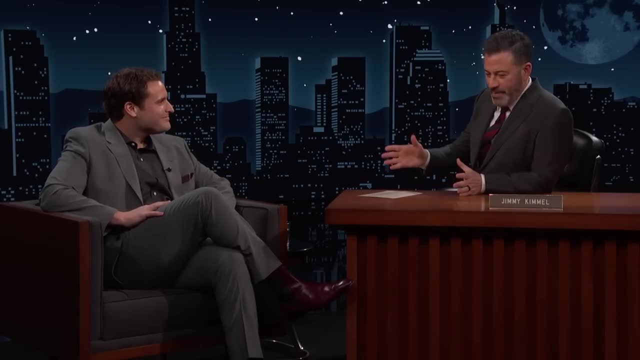 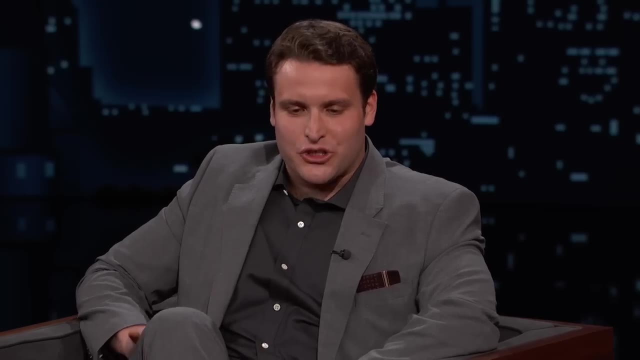 Not yet. yeah, I haven't gotten that far. You, when we met, was some kind of like gosh well, I don't exactly remember what happened. Your mom asked me to do something. Sure, yeah, It was. it was when my life peaked. 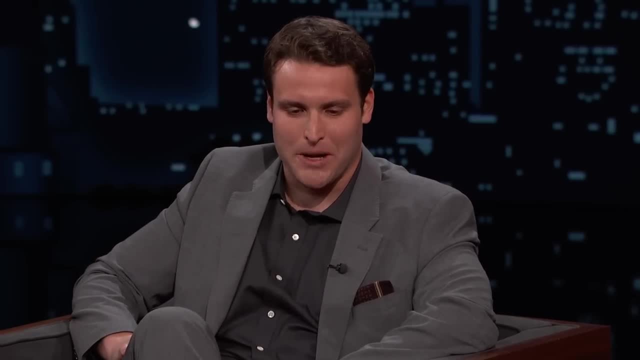 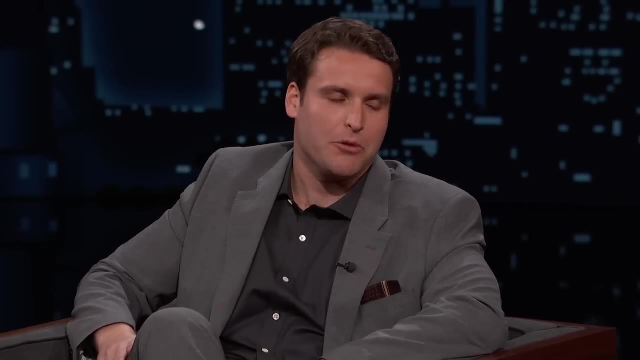 basically is when we met last. I'll go I'll give the full rigmarole of the story, but basically so at my high school we had this: you know a whole senior prank thing. right, You know, you come up with a senior prank. 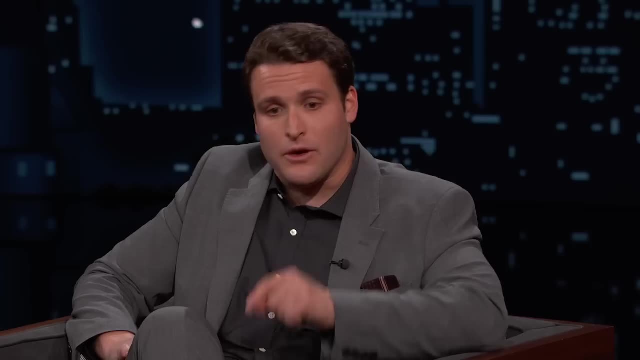 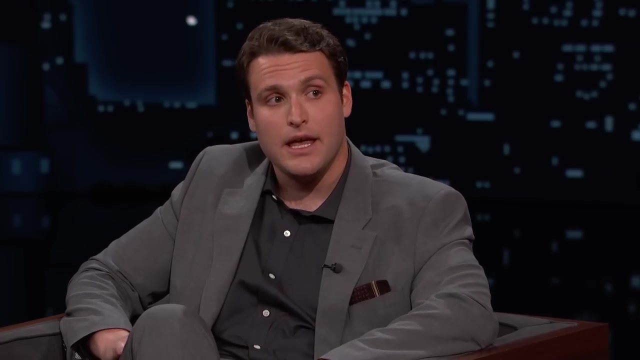 to do on the whole school. whatever, My friend Zach and I thought the greatest senior prank that we could ever possibly do would be to figure out a way to get you to come to campus and get in a physical fight with one of us. that was like choreographed in some way, right. 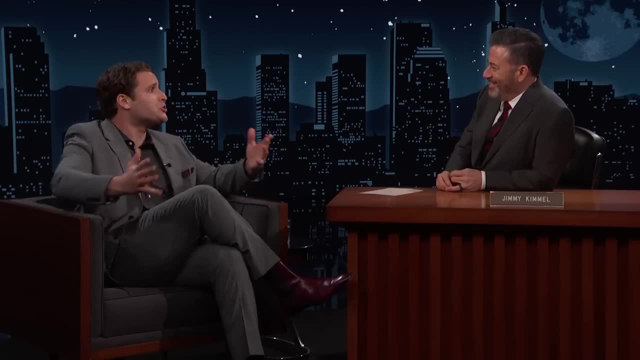 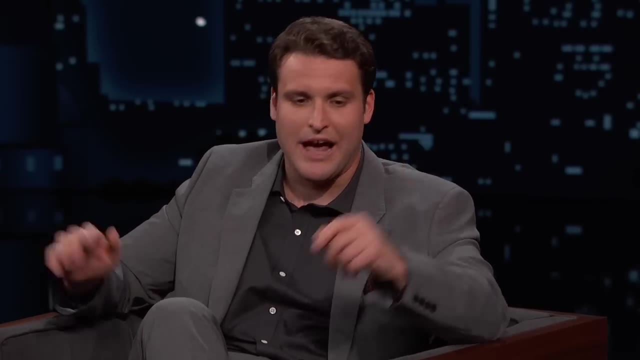 That would really be insane and the funniest thing ever. Maybe Matt Damon could show up. you know you guys could go at it, whatever. And then my mom comes on the show and she brings it up to you. She said: you know you have a laugh, whatever. 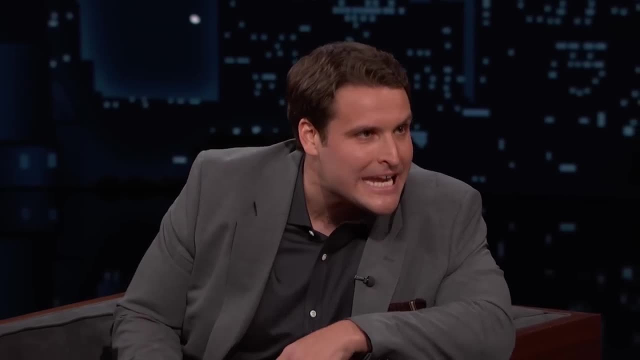 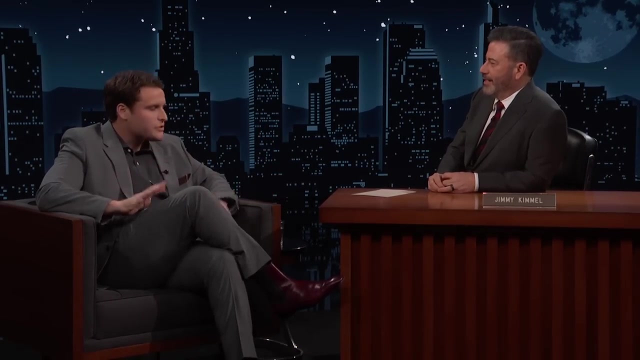 And then at the commercial break, you turn to her and go: I need to do this, Like you were completely down in every way, Like you had, you wanted to be a part of it, Yeah, yeah. So anyway, cut to. a few months later. 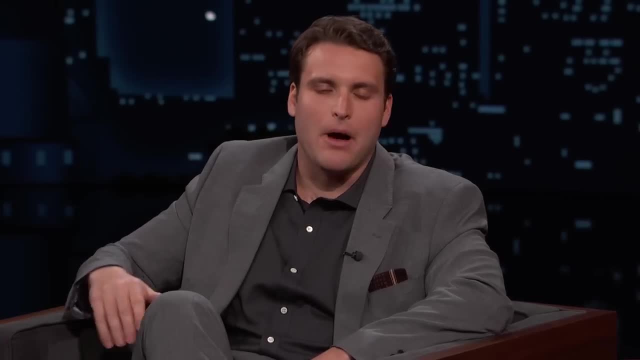 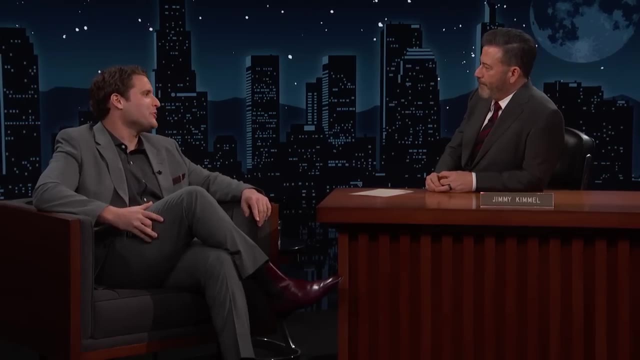 It's our senior grad night, right? And my mom had said: maybe you know we don't have you fight a minor at a school. Yeah, oh, we have to fight a minor. We don't want you to be put in jail. 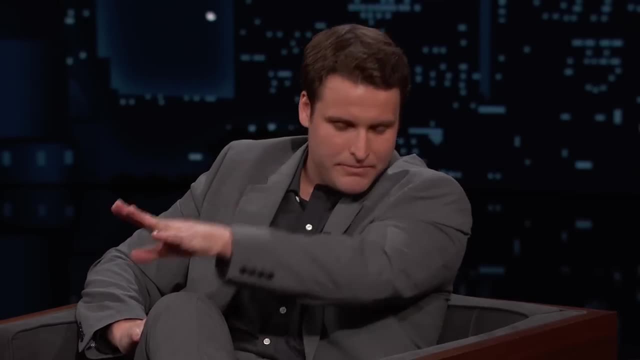 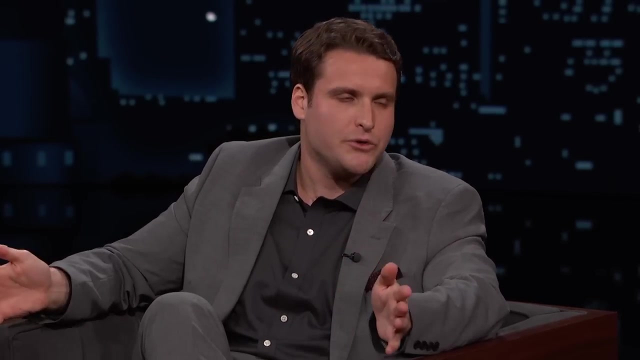 So anyway, so the fighting idea was kiboshed: Senior grad night, which is like the graduation night. They bring all the kids to some events so they don't go too crazy on the night that they graduate. whatever, We go to a Groundlings show. 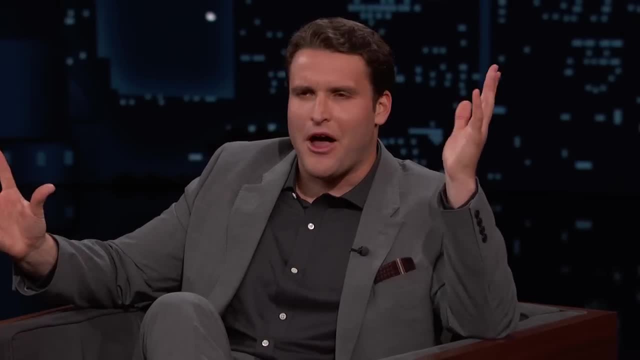 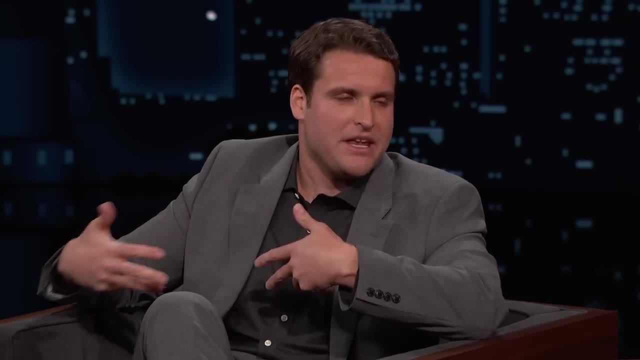 It's an improv group here in LA And it's great fun. They're doing all these awesome sketches and stuff, And then one of the sketches is for some kids to come up and be interviewed on stage, right, But the guy's in a bear costume, so they had this. 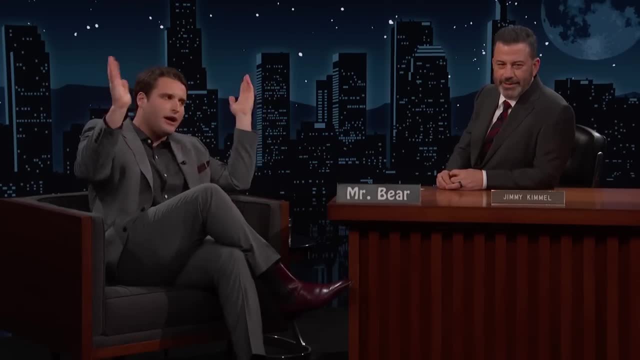 On the front, like you know, that type of Mr Bear right? Oh, he's going to interview. oh, that's so funny. whatever He pulls out a name from the story, Is this the real sign from then? 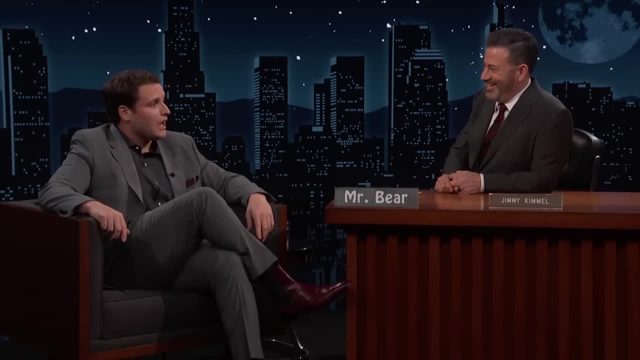 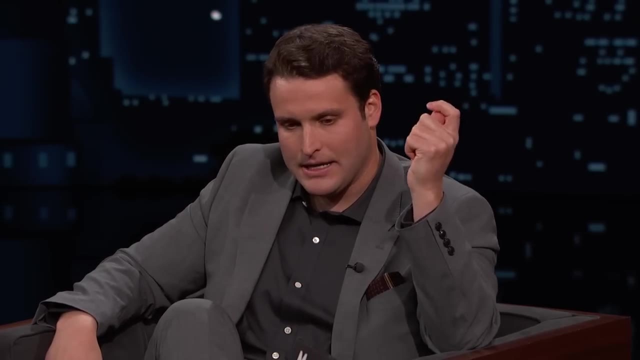 I have had this since that day. Oh wow, It's stayed with me, yeah, So, anyway. so the guy's using a bear costume, right, And he picks a name out of a hat And it's my name And the whole grade goes crazy. 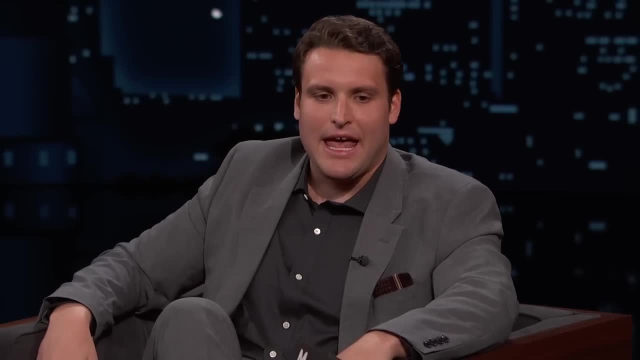 Oh Henry, oh my god, like you're going up there. So I go up on stage And I'm about to be interviewed by this guy in a bear suit And he says: oh, I forgot My hat, my bear head right. 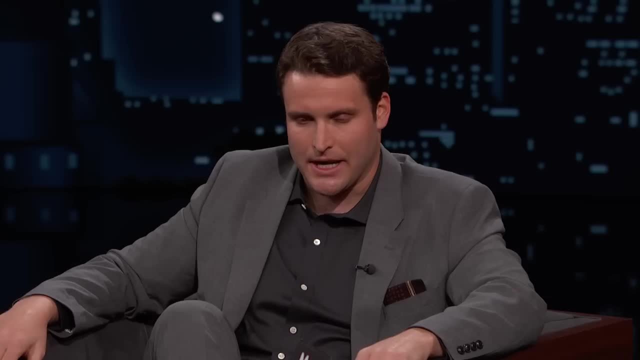 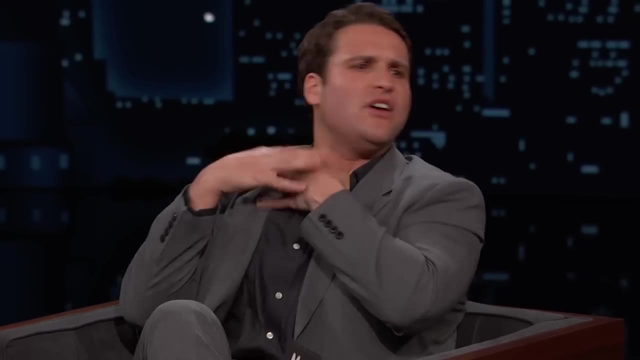 And he leaves. So I'm sitting there on stage alone for like a good 15 seconds And all of a sudden, out of nowhere, I feel like an arm around my neck like this. It's like a fuzzy arm. 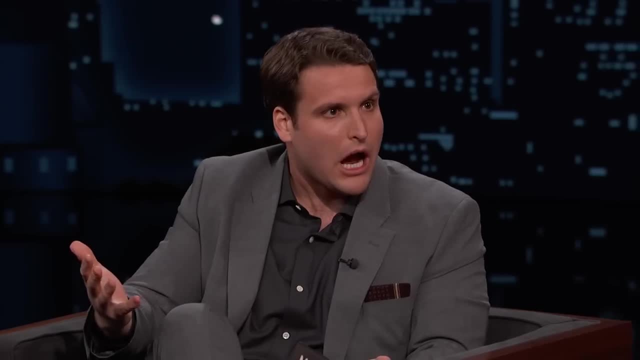 I'm like what the I get out of it? And it's this guy in a full bear costume. I'm like what the hell? And he goes. are you ready to fight a bear Like that? I'm like, uh, I guess. 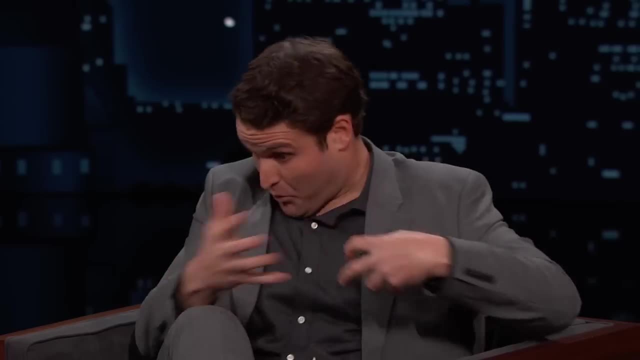 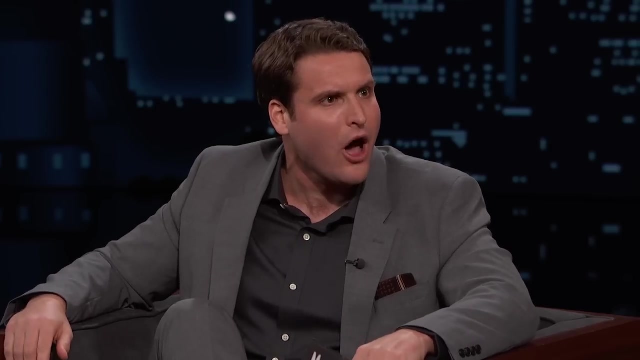 And we start wrestling on stage fully, really, you know, grappling wrestling on stage, right, Right, yeah. And then the guy starts going: pull my head off, Pull my head off, Like that. I'm like what is going on? 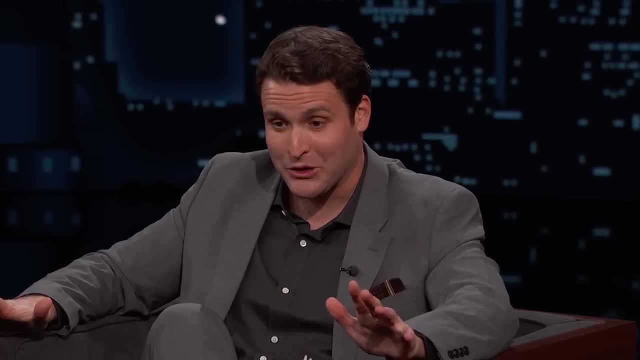 It was the craziest thing that had ever happened to me in my entire life And it was about to get crazier, because I pull the head off And we separate, And I'm panting like this And I look up. 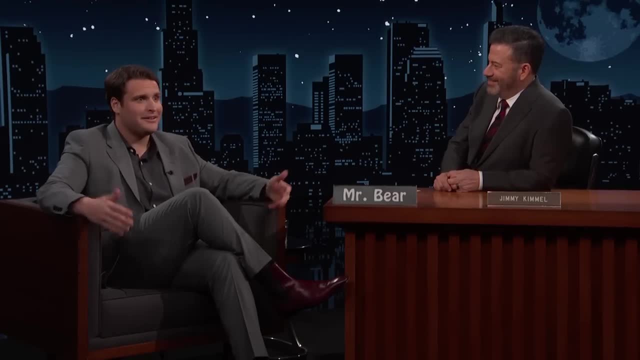 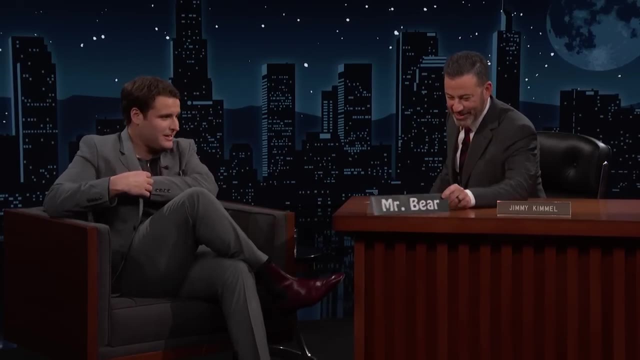 And it's Jimmy Kimmel, That's right. It was me So nice, Come on. When I came out as a furry- Yeah, I have a photo- And then we turned the thing around, right, And then it was like: 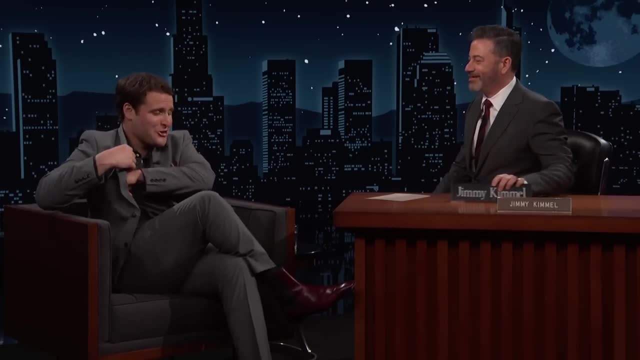 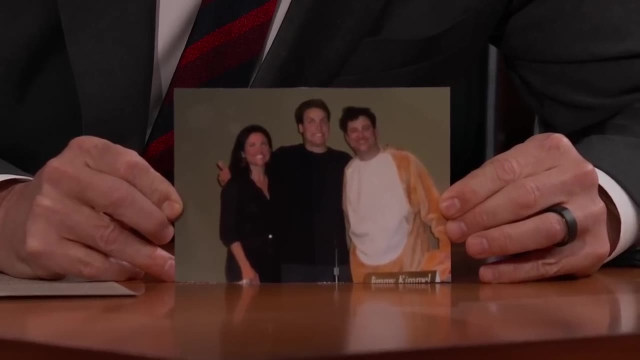 Yeah, yeah, One of those Big reveal. Oh, you have a photo of it? Yeah, I sure do. Oh yeah, Well, that's OK. So there we are. Oh, a real photo. OK, Let me show that, which is: oh yeah, there you go, yeah. 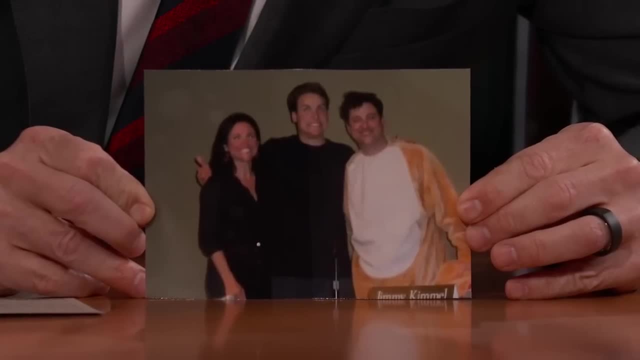 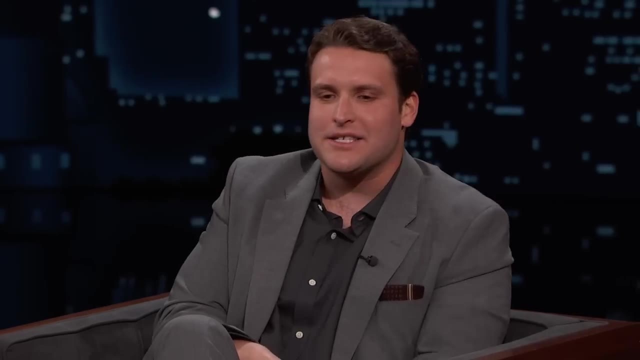 You're holding the head. The head was removed. Wow, yes, Annie Leibovitz took this picture. Well, it's good to. I mean honestly, man like you are the greatest sport. Well, the truth is, I'm in love with your mother. 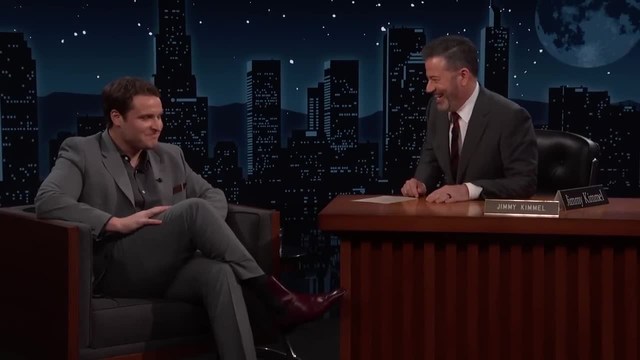 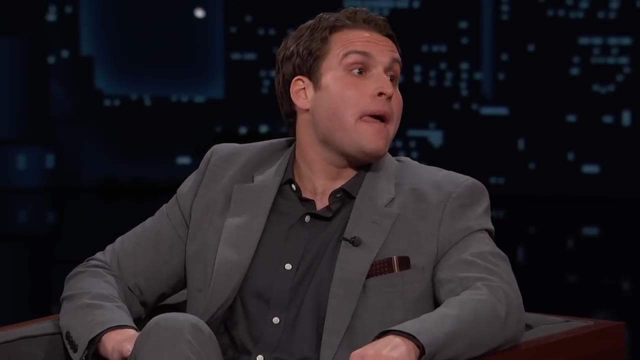 But that's really a Yeah. yeah, If you want to really know why I volunteered, I thought it was some weird sex thing she'd concocted. Oh OK, Turned out to be really weird. It was great to see you, man. 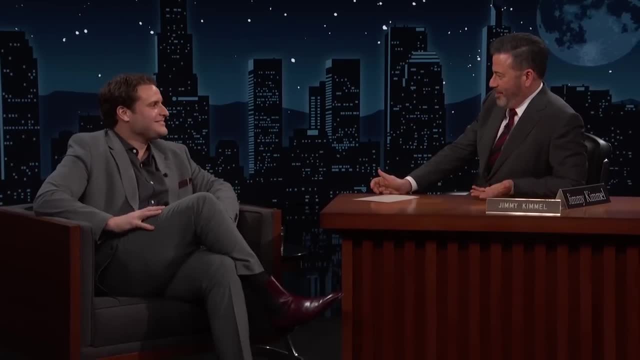 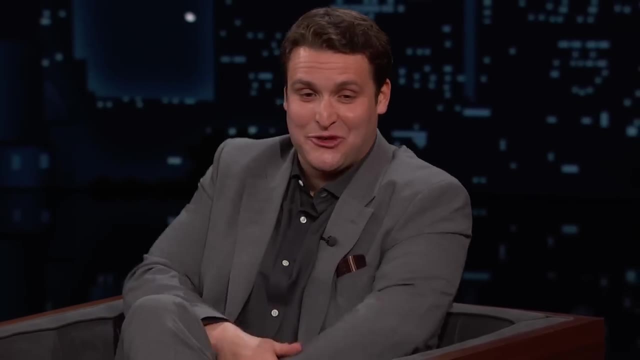 I'm taking off. Yeah, that's great. Yeah, And now you have your own show, which has got to be exciting and also maybe overwhelming. Yeah, I mean, it's a whirlwind Like I never. you know. I got this role kind of out. 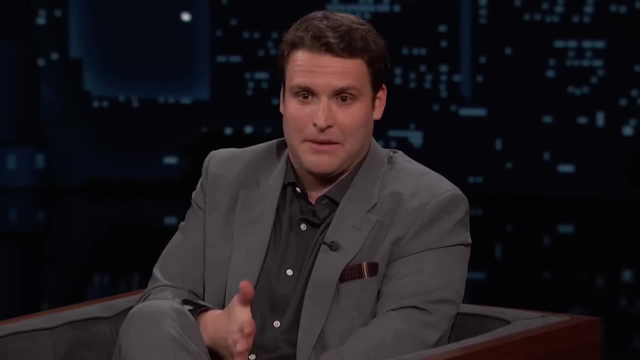 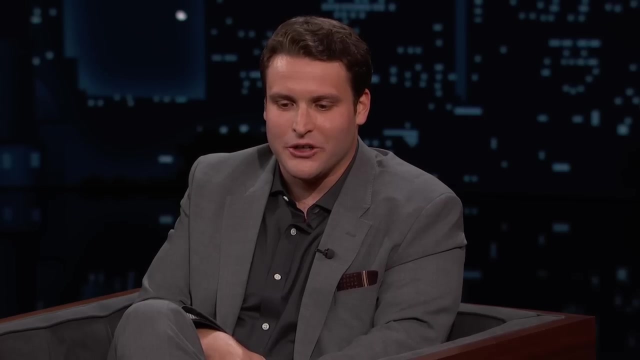 of nowhere, and I'd never been in something this big in my entire life. You were in a Curb, Your Enthusiasm episode. right, I was in a Curb episode. Yeah, yeah, yeah, Very lucky to have been in a Curb episode. 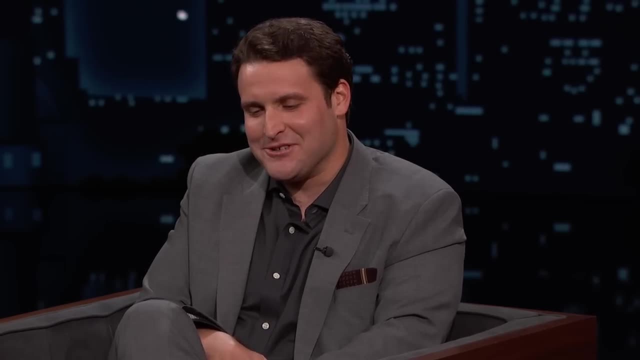 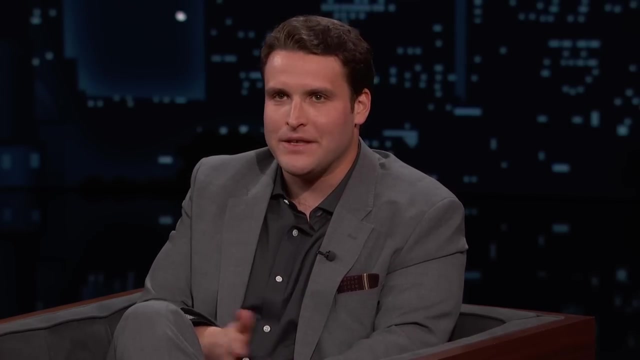 Now the show's over, which is very sad. Yeah, yeah, Yeah, that was a frickin' dream come true, And I well, so I'm in this episode. I play a fireman or something- paramedic. 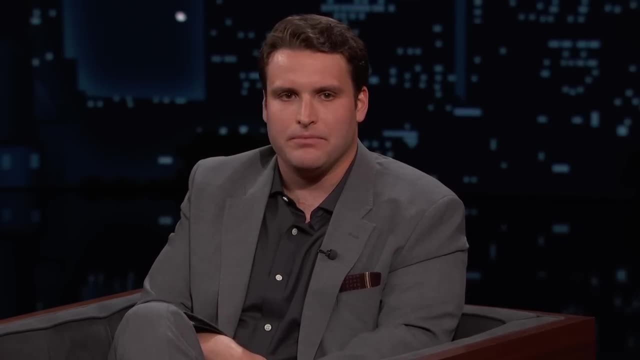 And it was my first real gig, right? So I'm like I want to soak up as much of this- Yeah, As much of this- as I possibly can. You know, I mean this is Curb Your Enthusiasm. 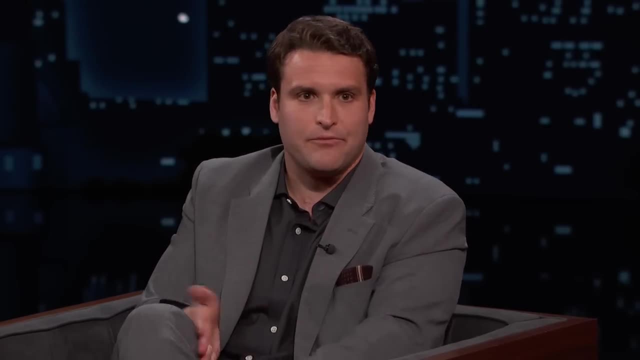 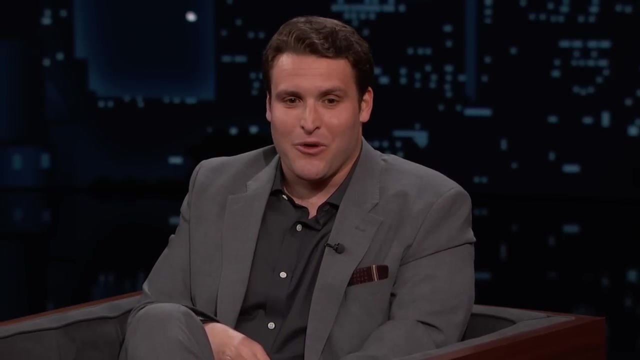 It's my favorite show of all time, the greatest ever, And I have a frickin' scene with Larry David. I mean what you know? it's a dream come true. So we do a take and we're going to do the next set up. 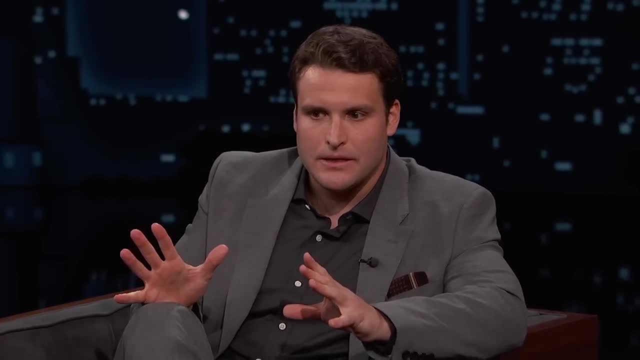 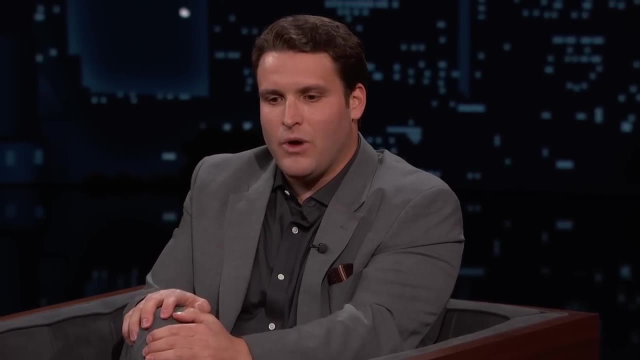 And I'm like, OK, I'm going to really, you know, see focus and see whatever you know, get, get. I'm behind the curtain, so to speak, right, I can really see what's going on and how the masters do it. 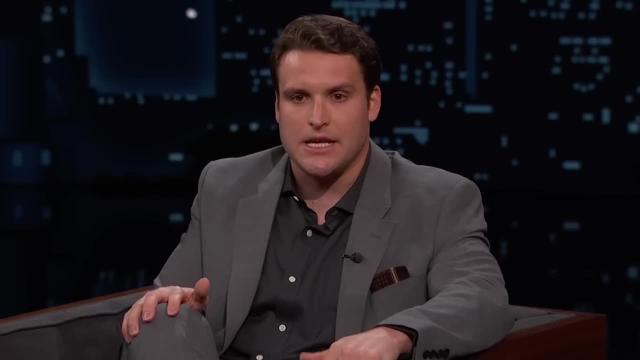 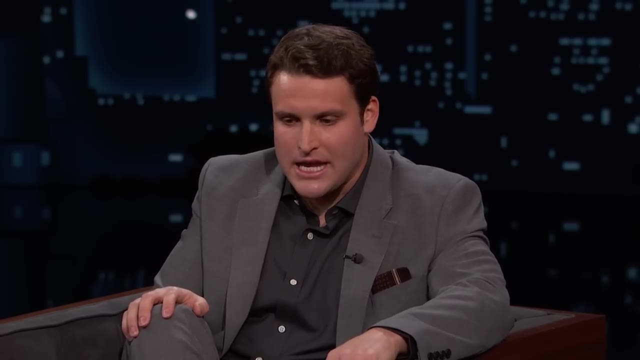 You know, and I'm like: oh, I wonder what Larry does between takes. I mean, he is the, he's the king, He's the greatest of all time, The GOAT, you know, the master of everything funny and the master of performance. 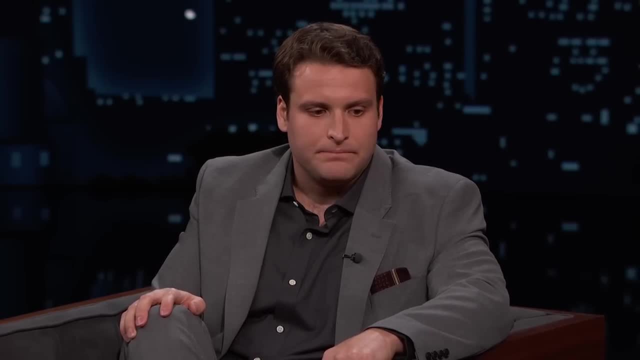 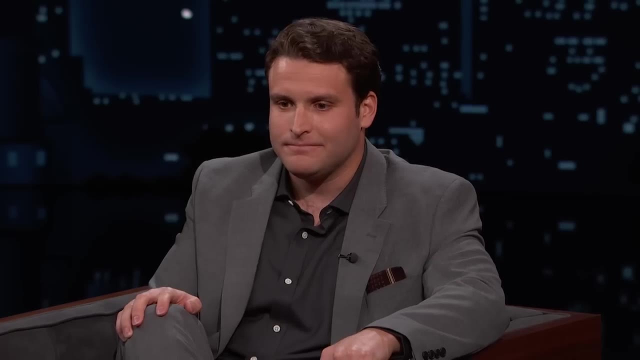 And I turn around to find him and he's practicing his golf swing. Yeah, he does that a lot, just practicing his golfing at nothing, Air swinging. and yeah, it was. I was like, OK, I can maybe relax a little bit. 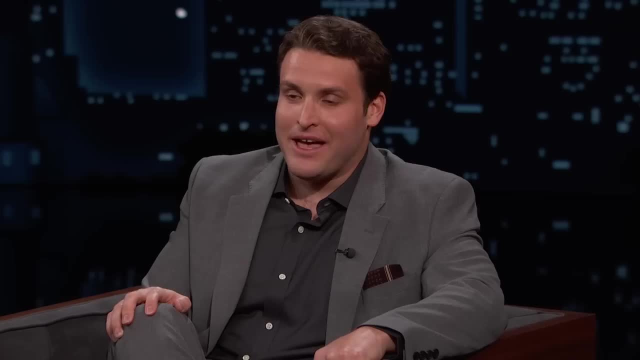 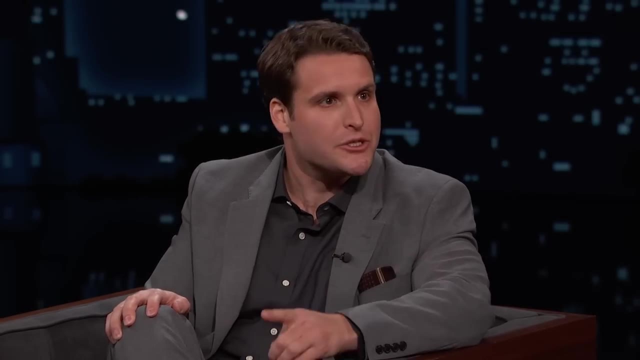 That's the lesson here. Who are your castmates on the new show? Oh man, The cast is really something. It's Michaela Watkins plays my mom, who actually she actually plays my mom's sister in some other projects. So that's like a weird, like web of fictional.